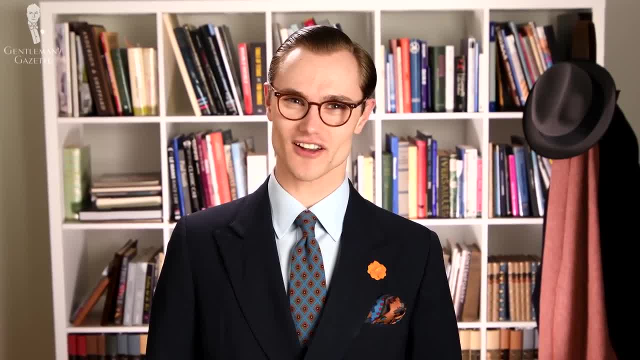 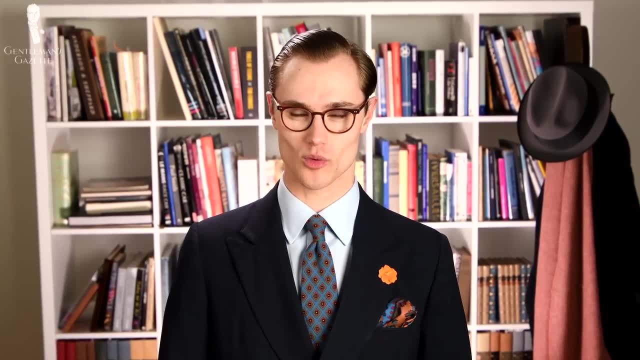 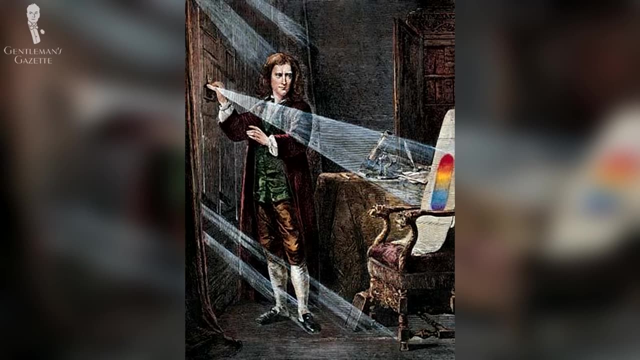 have to be a challenge. With that in mind, let's cover the fundamental knowledge you'll need to commit to memory in order to start experimenting. That is how to understand the color wheel, First pioneered by Sir Isaac Newton around 1665 to show the colors refracted from a beam of light. 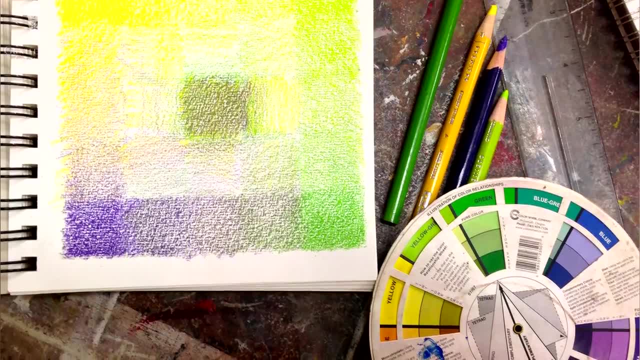 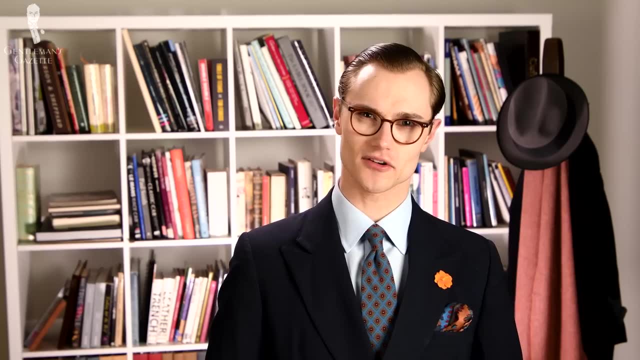 the concept of putting the colors of the rainbow in a circular orientation was soon applied to pigments as well. Thus the modern color wheel was born. In order to start discussing the color wheel, then we'll first turn to primary colors: The world. 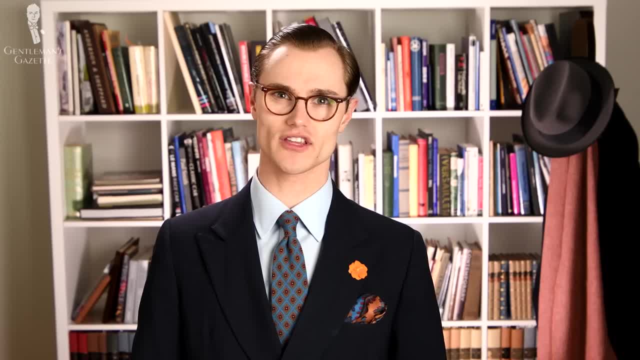 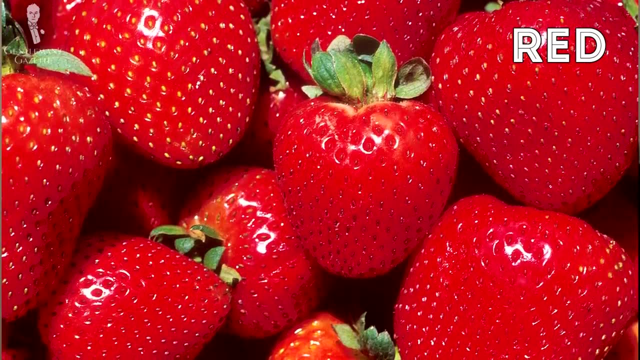 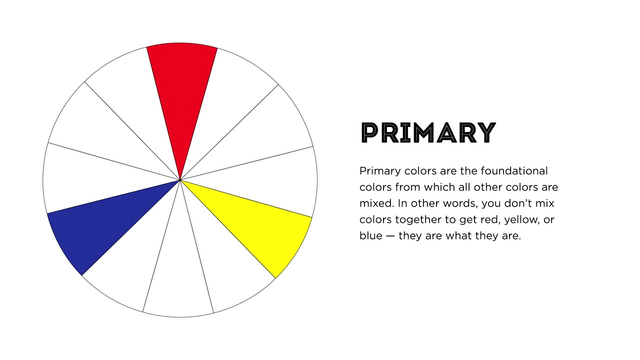 of menswear mainly concerns itself with the color wheel used in the visual arts. As such, the three colors we consider to be primary are red, yellow and blue. What is a primary color, then? Simply stated, primary colors are the foundational colors from which all other colors are mixed. In other words, you don't mix any. 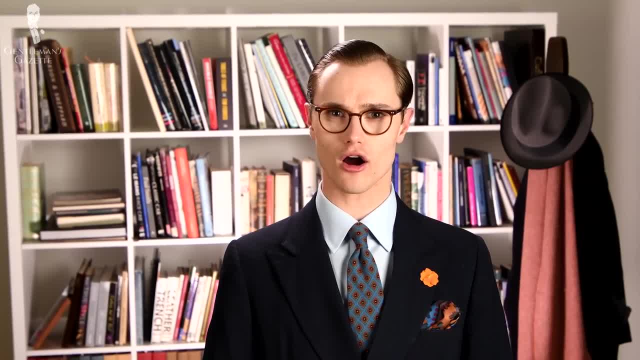 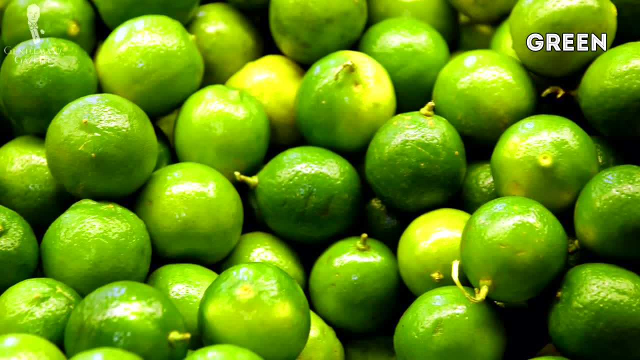 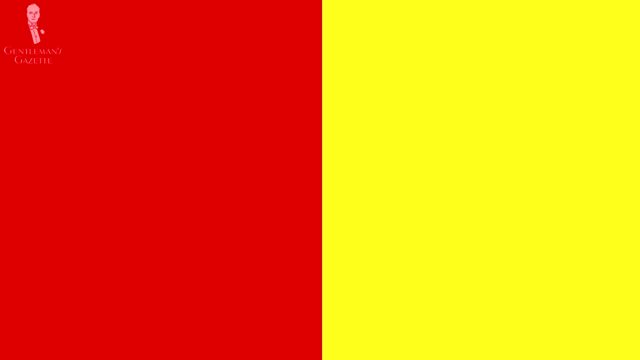 colors to get red, yellow or blue. They simply are what they are. Next up are the three secondary colors: Purple, also called violet, green and orange. The secondary colors are made by mixing two primary colors together, For example red. 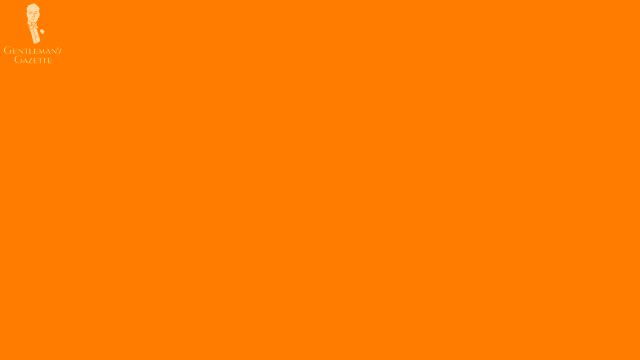 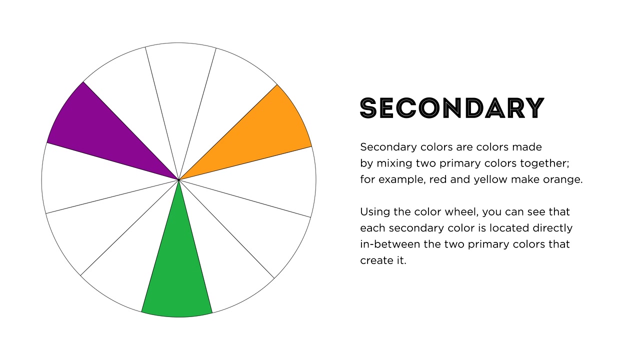 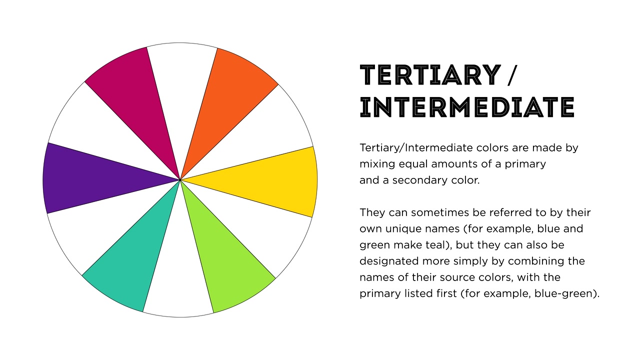 and yellow Combine to make orange. Referring again to the diagram of the color wheel, you can see that each secondary color is located directly in between the two primary colors that make it up. The final colors on the color wheel are intermediate colors, also called tertiary colors. They're made by mixing a primary 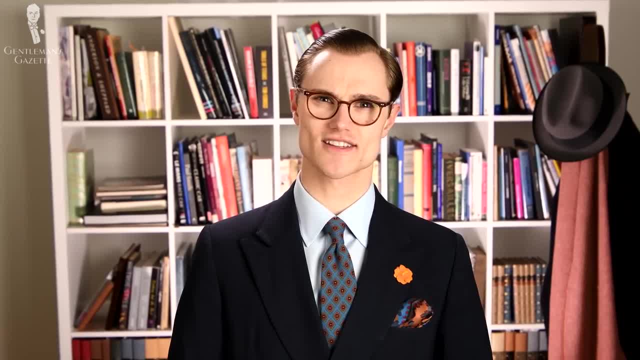 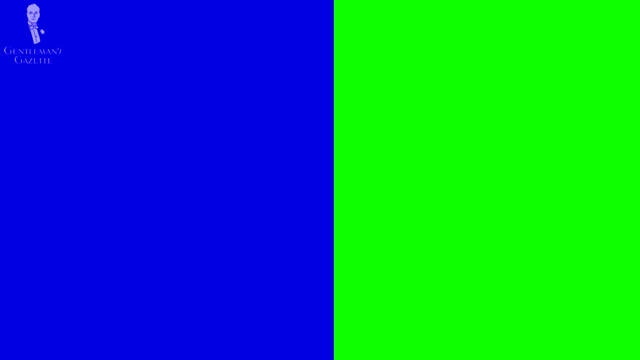 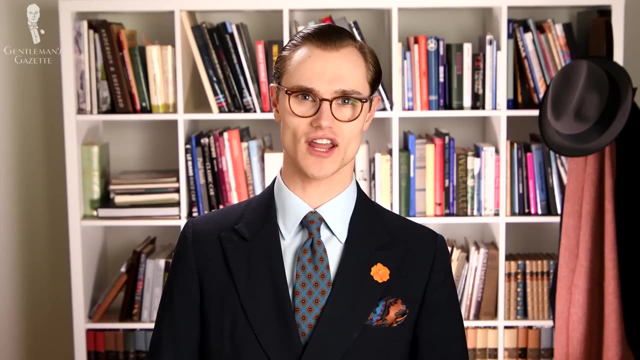 color and a secondary color together. These colors can sometimes be referred to by their own unique names. For example, the combination of blue, blue and green can sometimes be called teal. but in more simple terms, they can also be referred to by simply combining the names of the colors that create them with the primary. 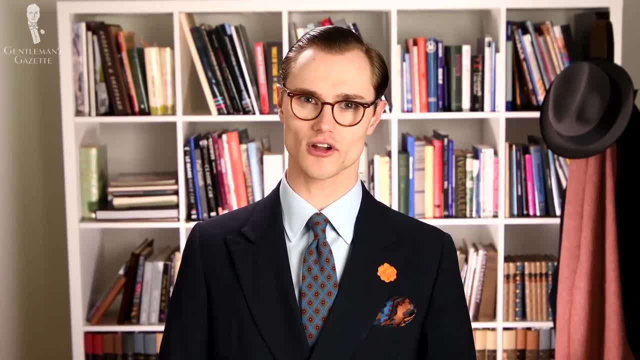 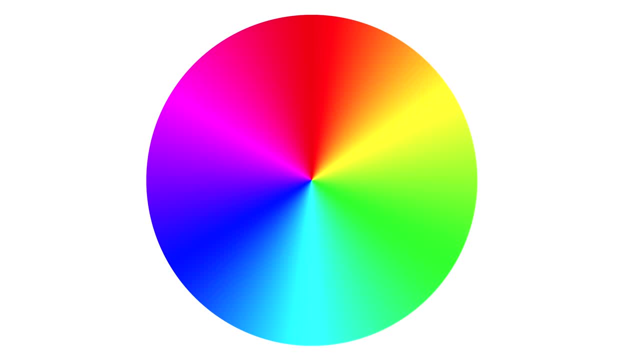 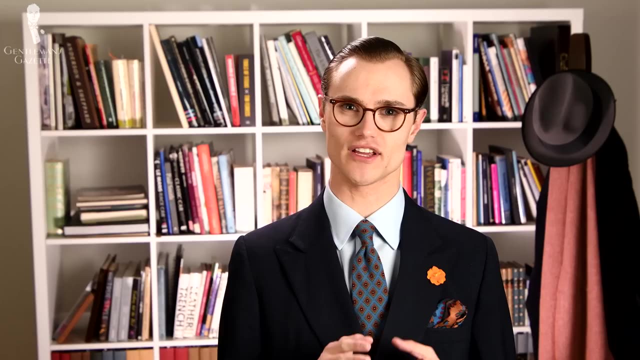 color coming first. So, for example, teal could also be called blue green. There are, of course, many thousands of variations in colors, each with their own specific names, but for the general purposes of color theory, breaking the color wheel down into 12 simple parts should be sufficient. 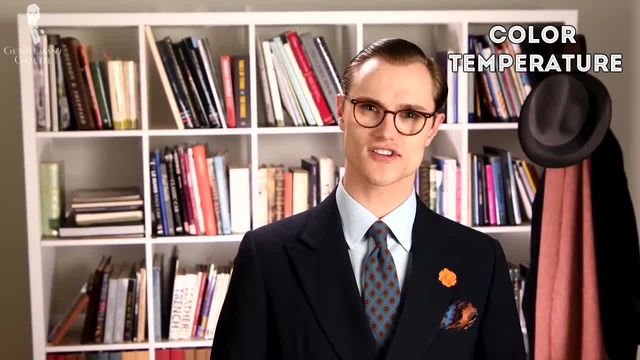 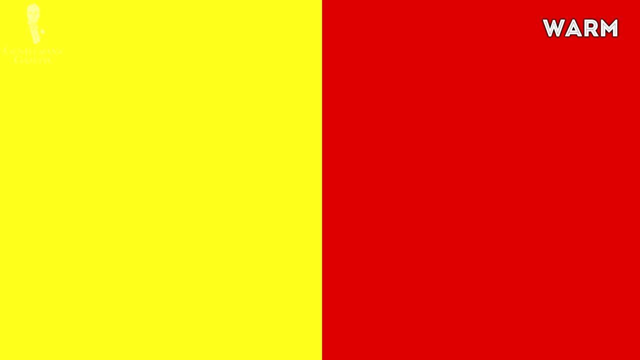 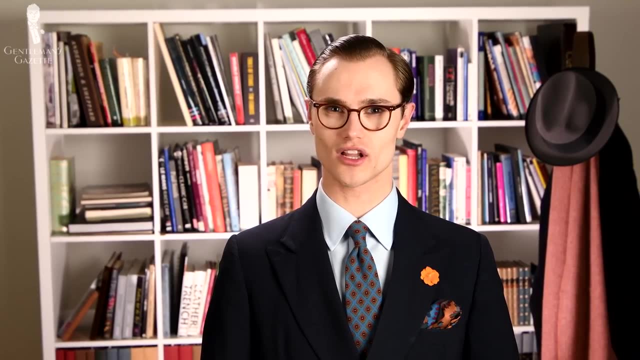 Next up, let's talk about color temperature, which refers to the perceived warmth of a color. Of the three primary colors, red and yellow are said to be warm, whereas blue is considered cool. It follows, then, that any combination of red and yellow will also, by default, be a warm. 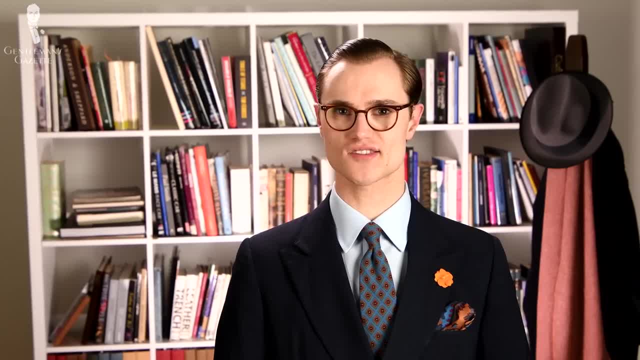 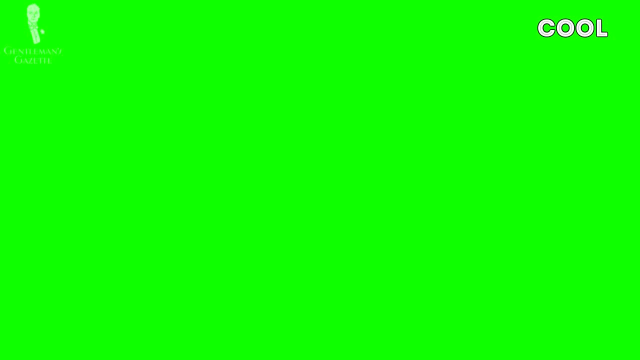 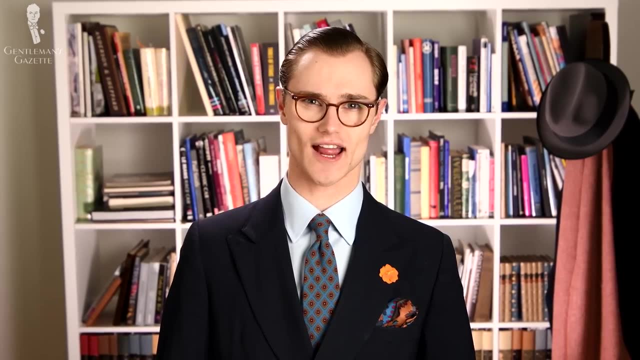 color. Meanwhile, when cool blue mixes with one of the warm primaries, different things result. While green is usually said to be a cool color, purple is often said to be a warm color. Even so, the relative temperatures of these secondary and intermediate colors can vary. 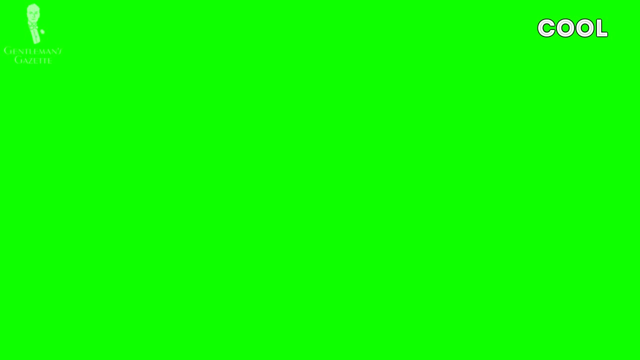 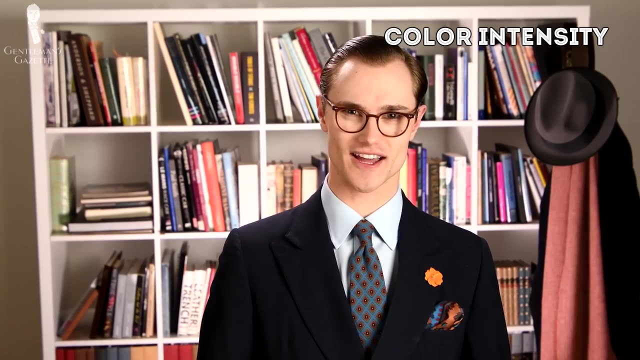 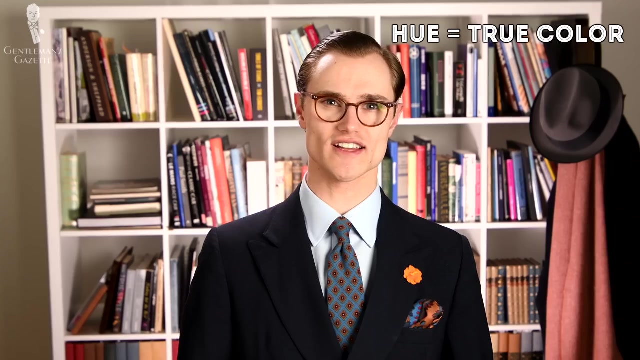 For example, while green is collectively considered to be cool, a yellow green will still be warmer than a blue green. Another important concept Understand is that of color intensity, or the lightness or darkness of a color. Another word for color is hue, and that's usually the word used when we're talking about the 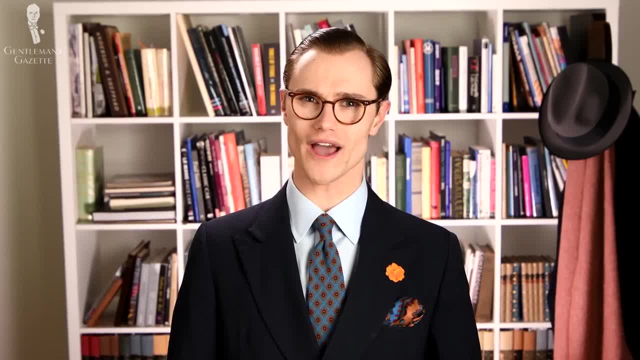 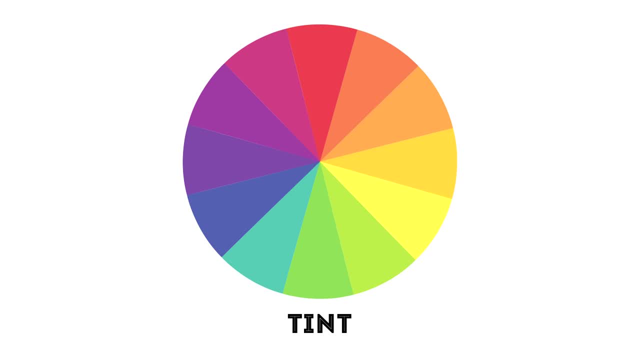 relative lightness or intensity of a color. If white is added to any color, this is referred to as a tint of that color. The result is a lighter and less intense hue. Conversely, if black is added to any color, this results in a shade. 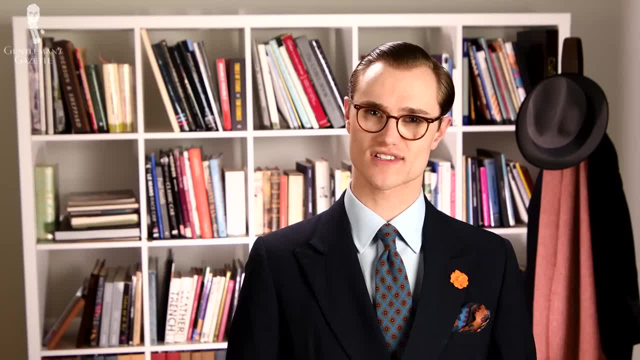 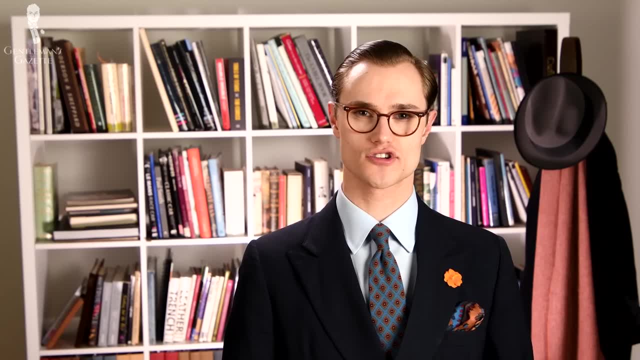 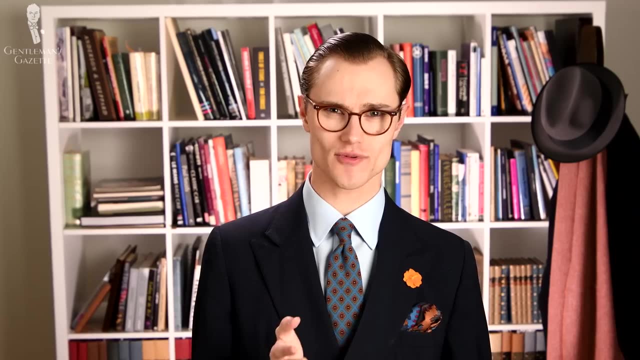 Sometimes also called a tone of that color. The result is darker and also less intense. For the highest intensity possible in a given color, just go with the default true hue. Speaking of black and white, they're not considered colors in the strictest sense, since they're. 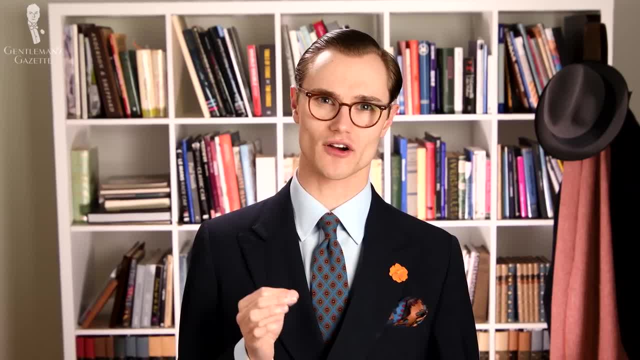 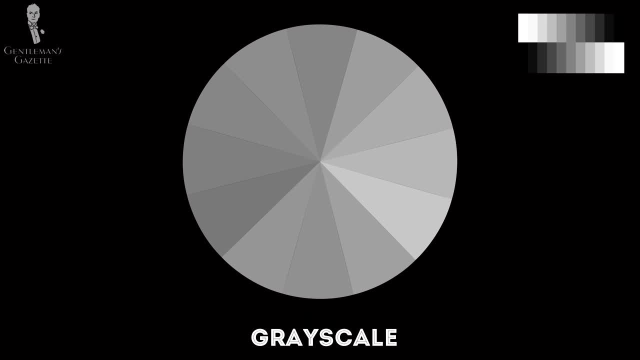 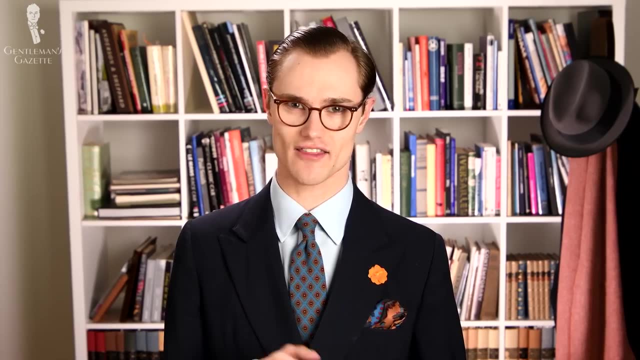 not on the color wheel. Rather, they reside on their own spectrum, which we refer to as the grayscale, since when black and white are mixed together in varying quantities, They result in different shades of gray. It's also sometimes said that you can achieve black by mixing together all of the colors. 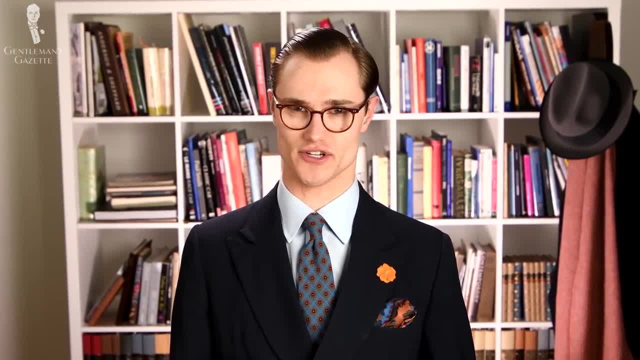 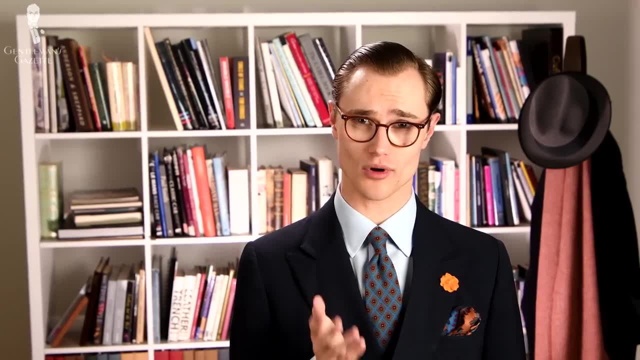 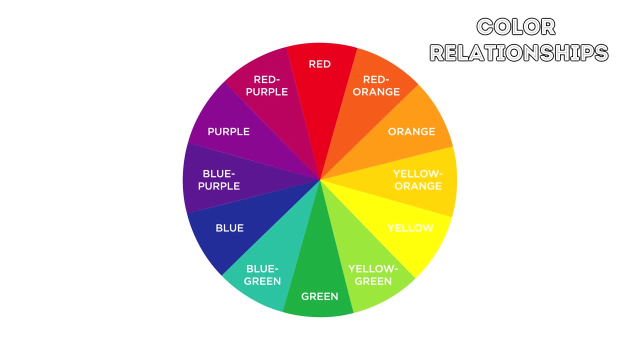 on the color wheel, though this is really more of an approximation. You may also have noticed that brown isn't anywhere to be found on the color wheel. This is because, in order to create a brown tone, certain colors have to be mixed together. This brings us to our next important point: color relationships. 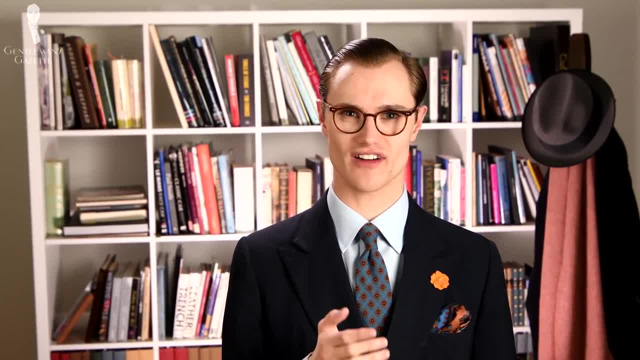 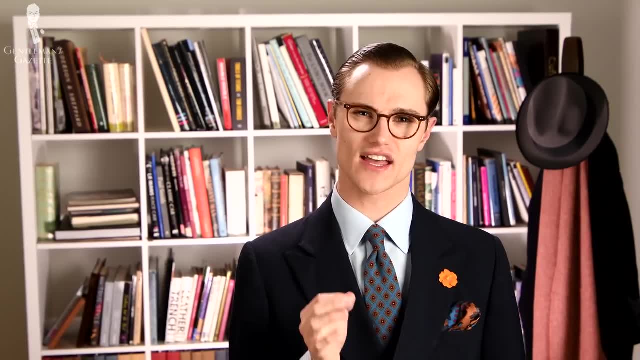 In addition to the colors on the wheel relating to each other In terms of how they mix together, they also have relationships in terms of how they interact when they're kept separate. If that's a little hard to understand, just keep your eye on the color wheel for these. 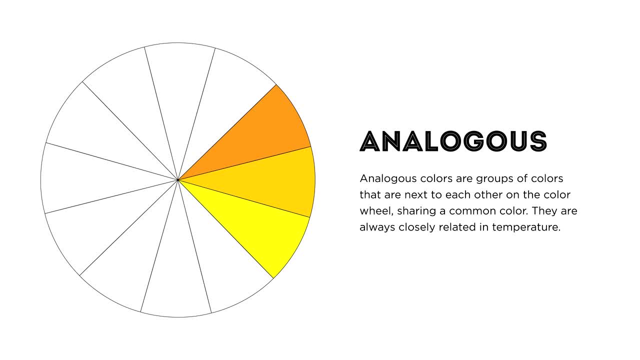 next few terms and everything should come together. The first term we'll go over for these kinds of relationships is analogous colors. Simply put, analogous colors are ones that are similar in temperature and are found close to each other, and sometimes directly adjacent, On the color wheel. any color analogous to a primary color is a color that features that. 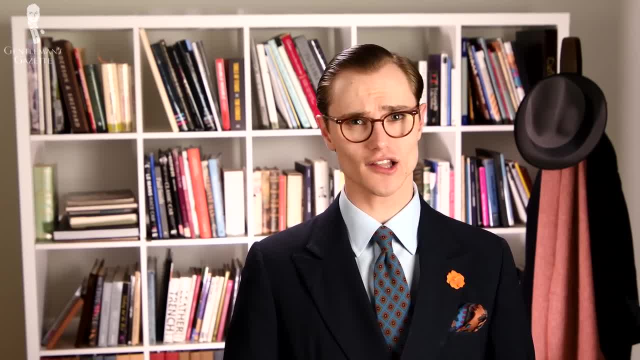 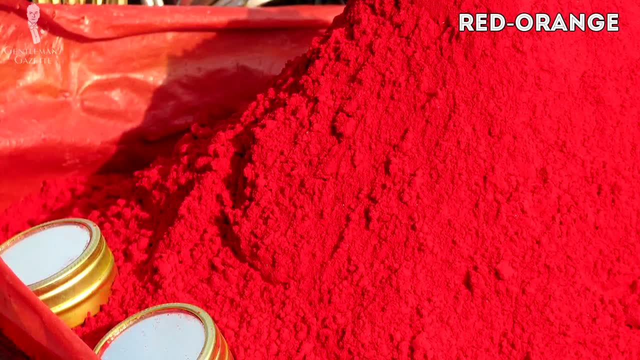 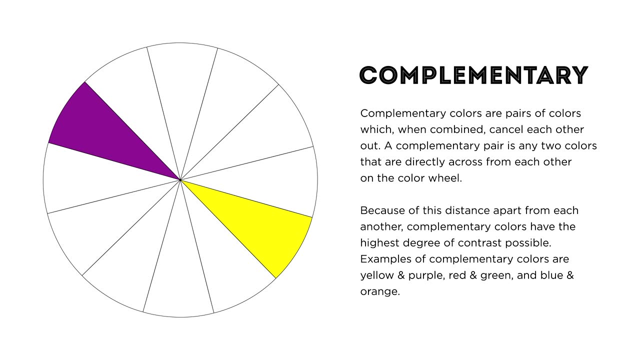 primary. So, for example, everything from yellow orange to red orange is analogous to yellow, because all of those colors feature some amount of yellow in them. The other important color relationship is that of complementary colors. In simplest terms, any two colors that are directly across from one another on the color. 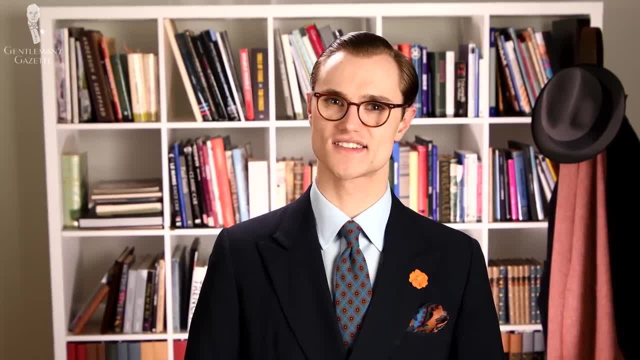 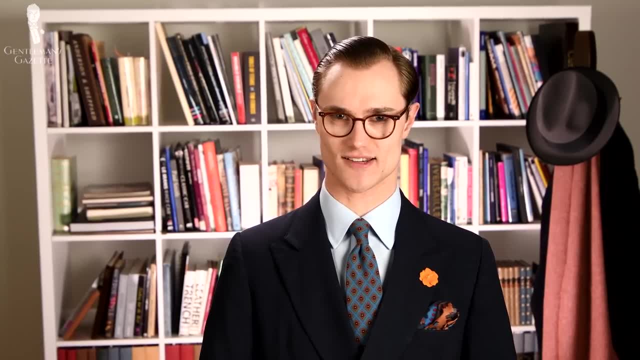 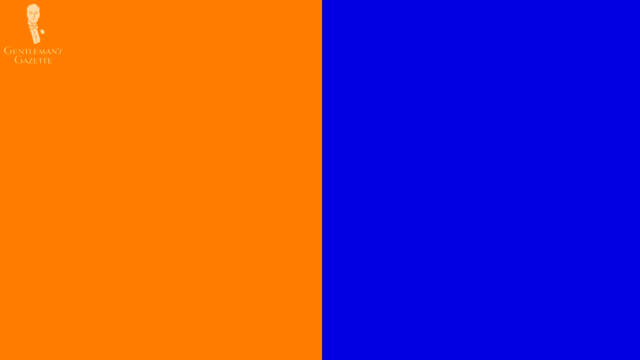 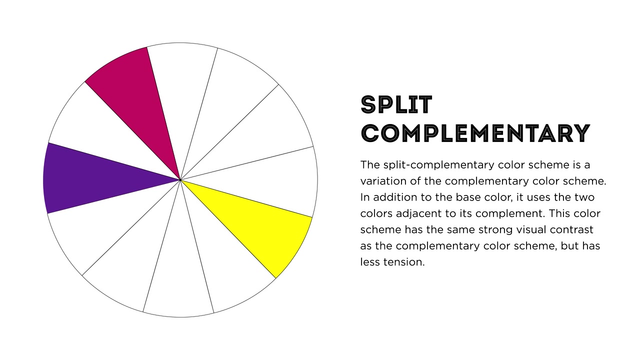 wheel are considered complementary Because of this distance apart from one another. on the color wheel, complementary colors have the highest amount of contrast possible. Some examples of complementary colors include red and green, yellow and purple and blue and orange. In addition, the designation of split complementary colors can be applied to any one color and 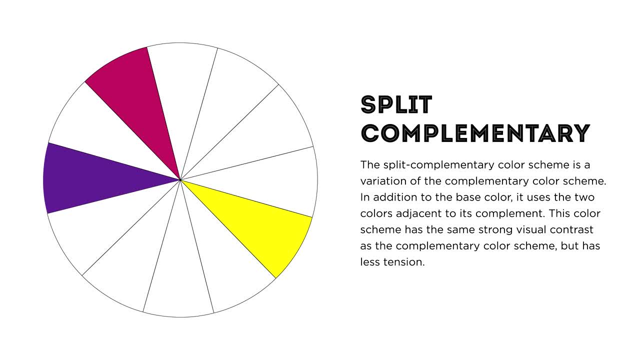 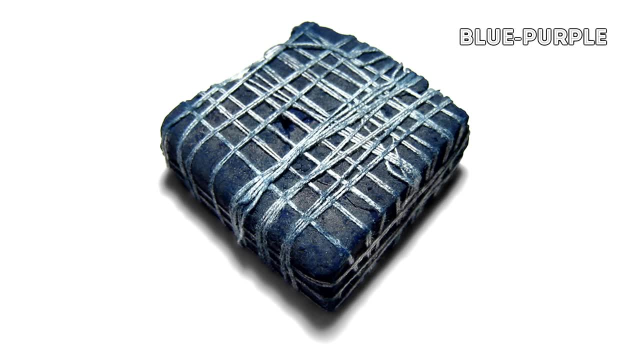 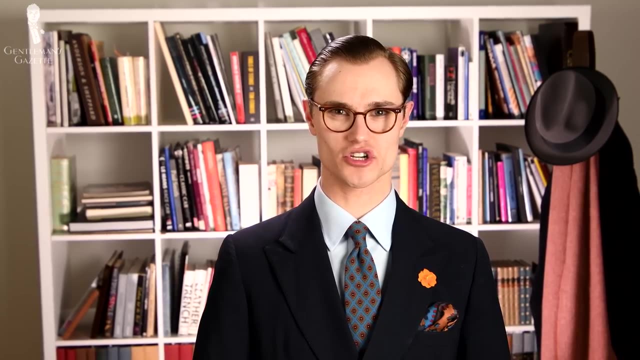 the two direct analogs of that color's complement. To state that more simply with an example from the color wheel: Red purple and blue purple are the split complementaries of yellow. So answering our question about how to get brown, then, the simplest way to achieve a 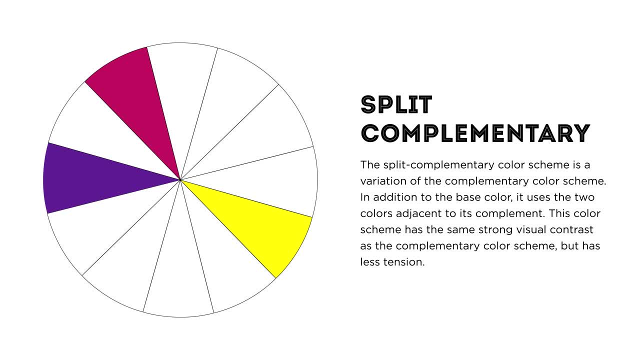 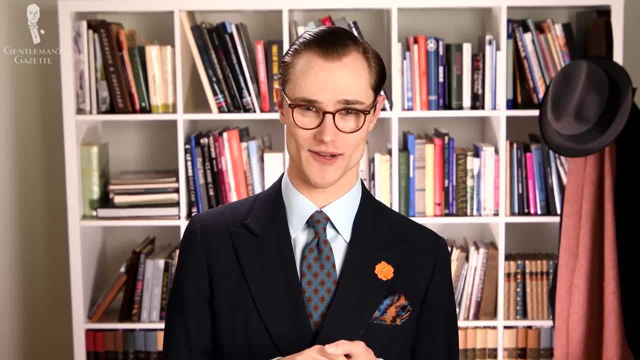 brown tone is to mix complementary or split complementary colors together. Simple, right, There's a complete overview of the color wheel out of the way. With all that knowledge at hand, you might now be asking the broader question: why is it important to understand color relationships in color? 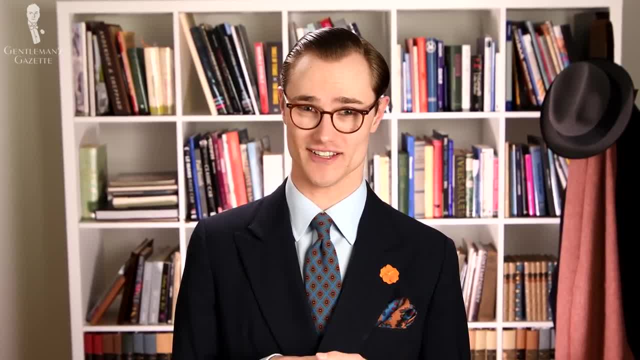 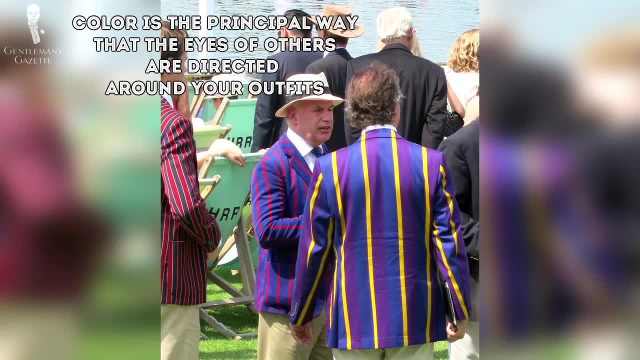 Why is it important to understand color relationships in color? Why is it important to understand color relationships in terms of putting together your outfits? The answer is because color is the principal way that we can direct the eyes of others. The primary objective of any colors in an outfit should be directing the eyes of the 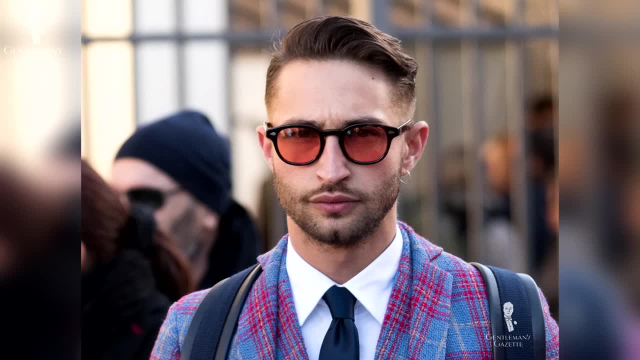 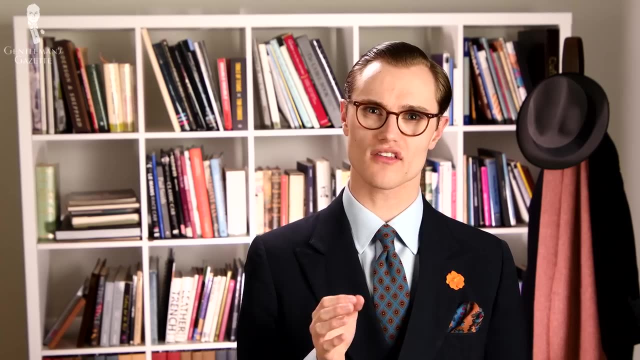 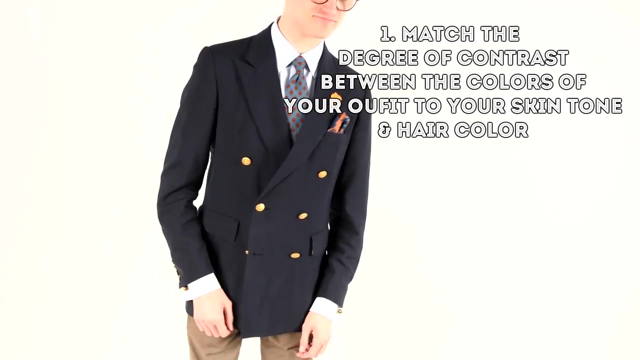 viewer to your face and also making your face look as well-colored and healthy as possible. What's the best way of going about doing that? In short, there are two main methods for achieving this effect with your outfits: 1. The first of these techniques is to match the degree of contrast between the colors. 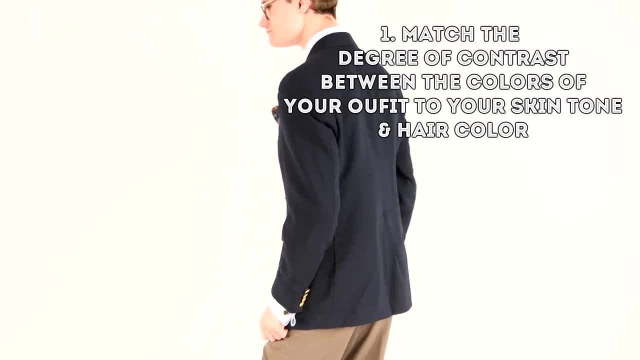 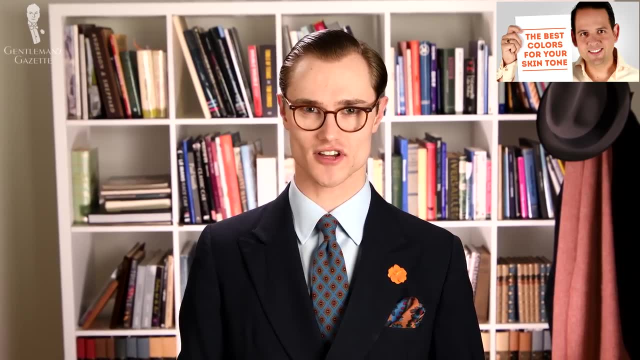 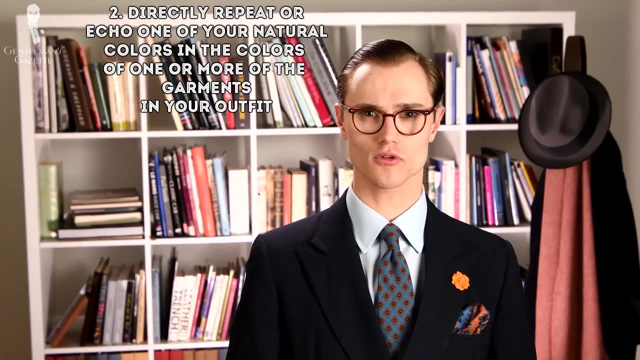 in your outfit to the degree of contrast between your skin tone and your hair color. Speaking of which, you can find our video on how to properly determine your skin tone here. The second technique is to directly repeat, or otherwise echo, one of your natural colors. 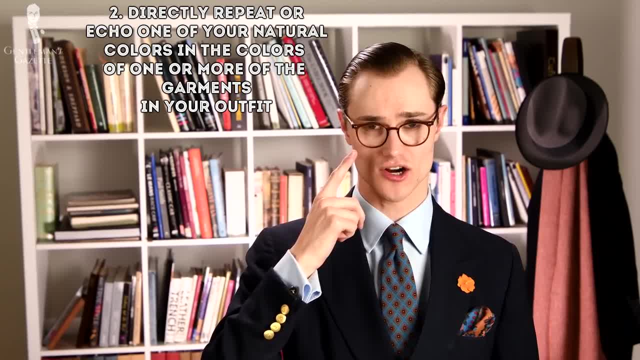 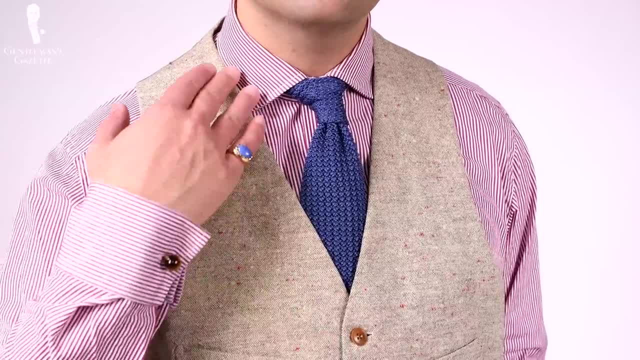 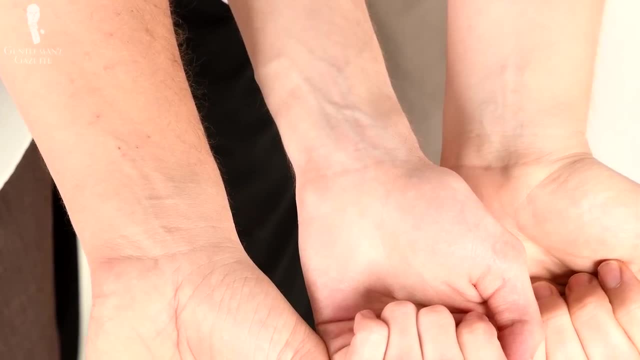 whether that be your skin tone, hair color or eye color, in the colors of one or more garments that make up your outfit. As such, here are our tips on how to wear and pair your colors effectively. Regarding the degree of contrast between a man's skin tone and his hair color, men fall. 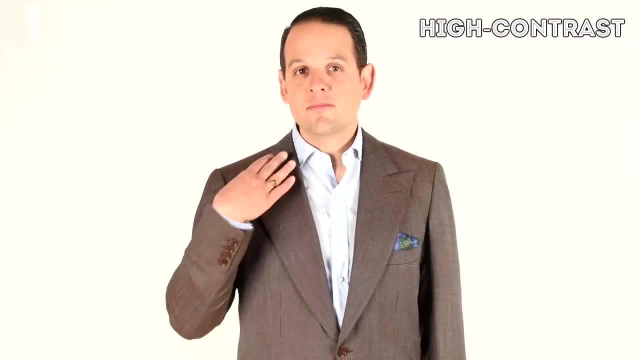 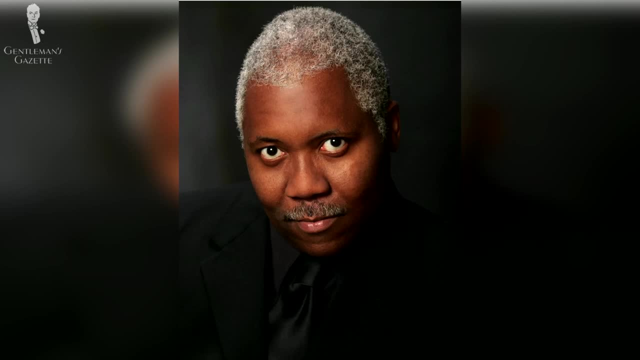 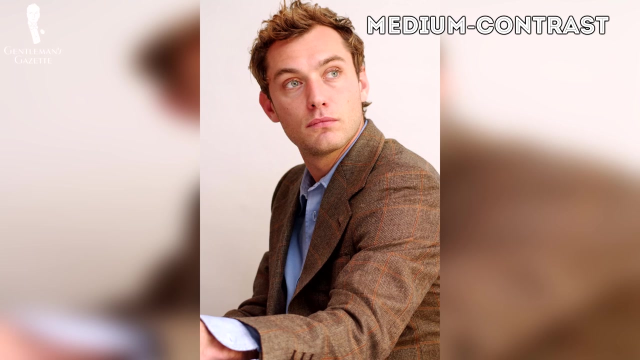 into one of three basic groups: High contrast, which is most typically characterized by fair skin and dark hair, though the reverse could also be true for darker skinned men with dyed or graying hair. medium contrast, where the colors are different But not to a large extent. and low contrast: either fair skin with blonde or graying hair. 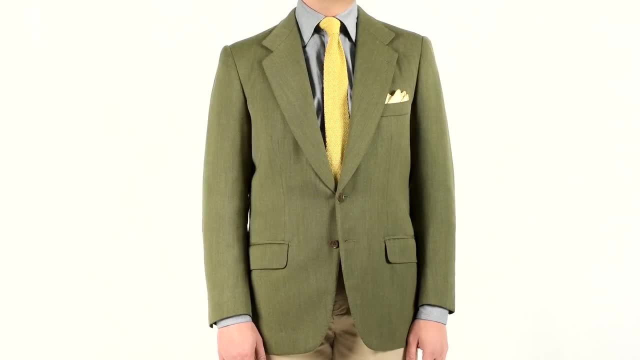 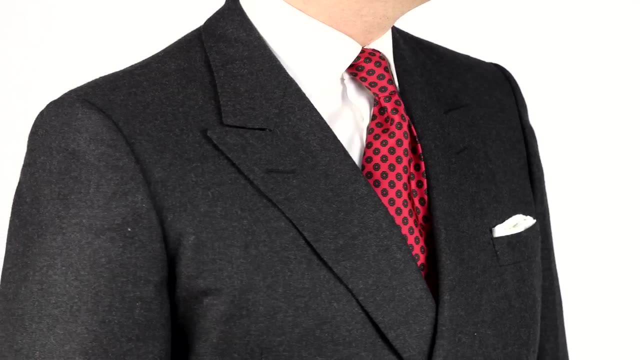 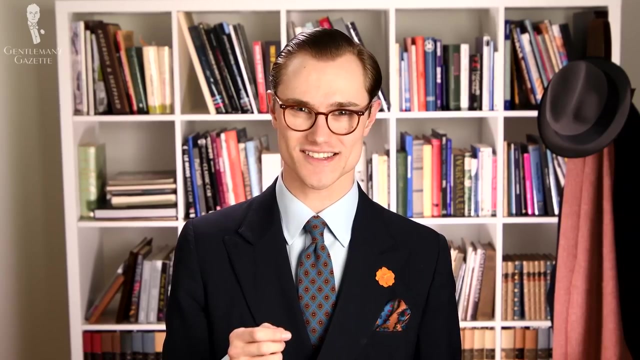 or dark skin with dark hair, High contrast men can more safely experiment with wearing combinations of bolder colors, For example pairing primaries or complementary colors together. Just don't go for the true hues of all of these colors when you're pairing them together. 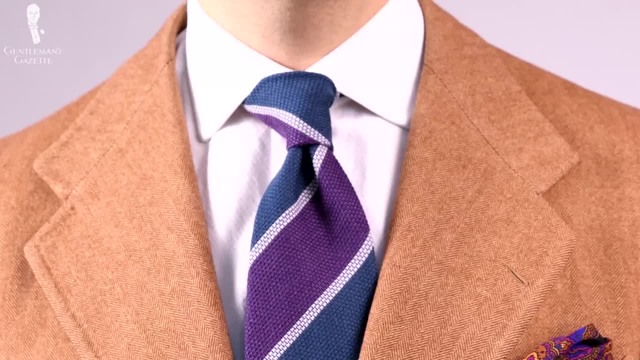 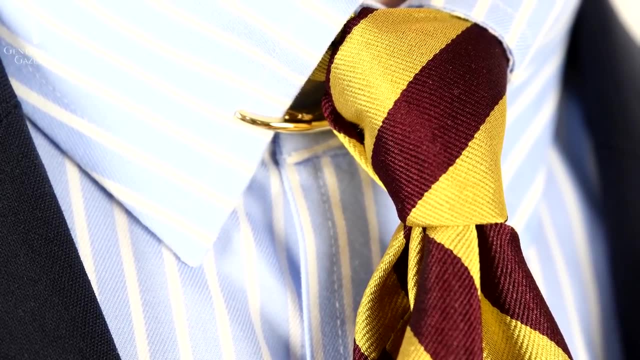 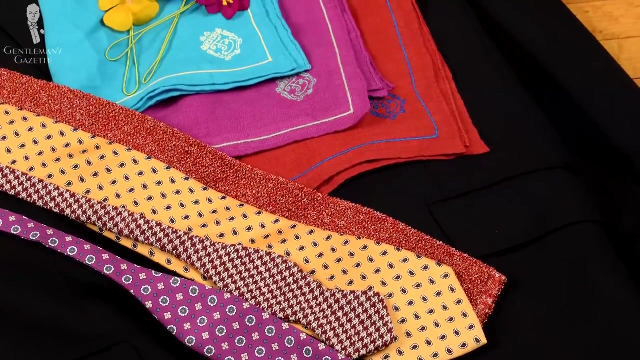 or you will fall into that trap of looking like a clown. Instead, try pairing primaries or complements that have been further augmented with tinting or shading. For example, you could wear a pastel blue shirt with a darker, burnt orange tie- A medium contrast. man can, of course, wear a garment that is bolder in color, but he should. 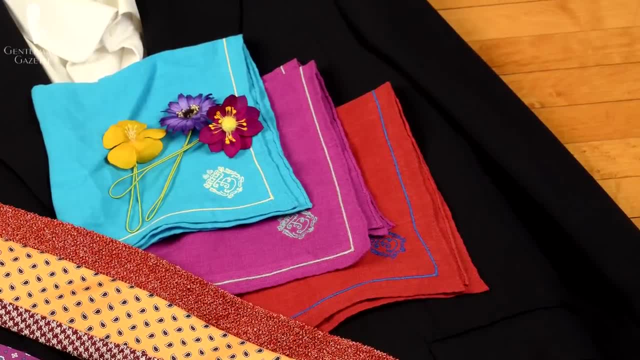 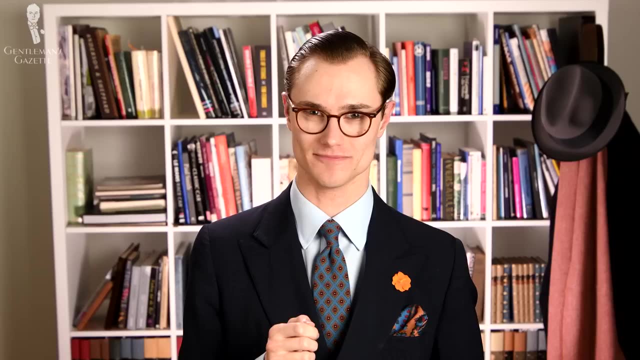 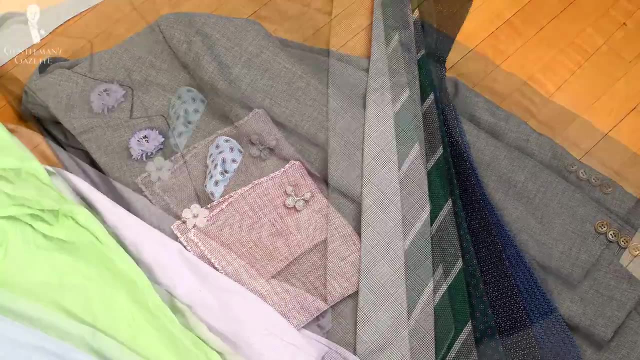 be mindful that if he does so, it will draw some attention away from his face. Again, as with many things in menswear, Confidence is key here. Low contrast men are the ones who should be most careful in pairing together contrasting colors. Really, make sure that you've muted the hues of the contrasting colors if you decide to. 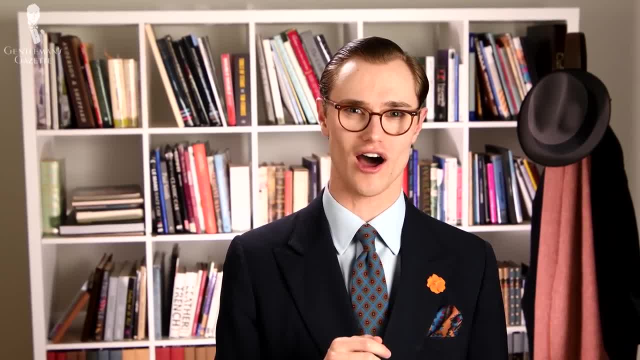 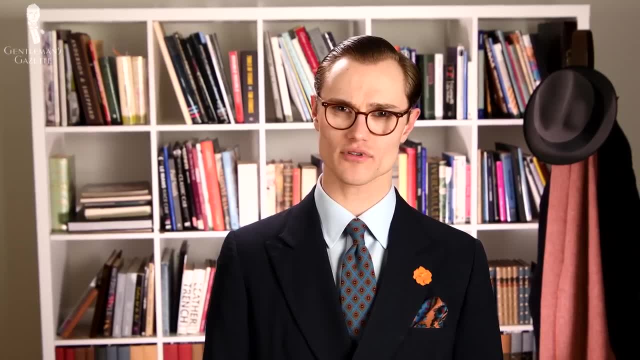 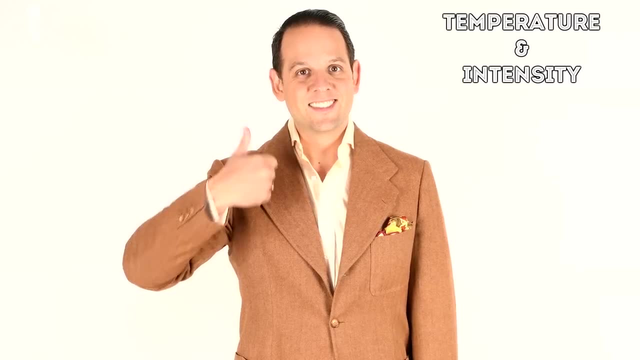 wear them, as that's the best way that you'll be able to pull them off. When it comes to having colors in an outfit that echo a man's natural tones, the keys here are temperature and intensity. We've covered this specific topic in depth in that video on how to find your specific. 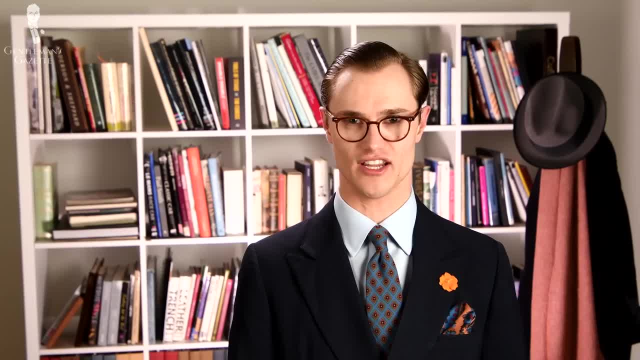 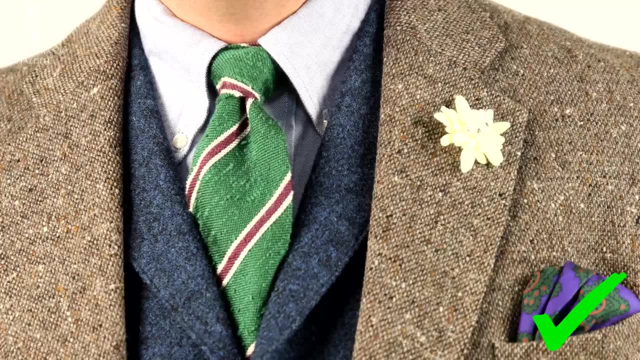 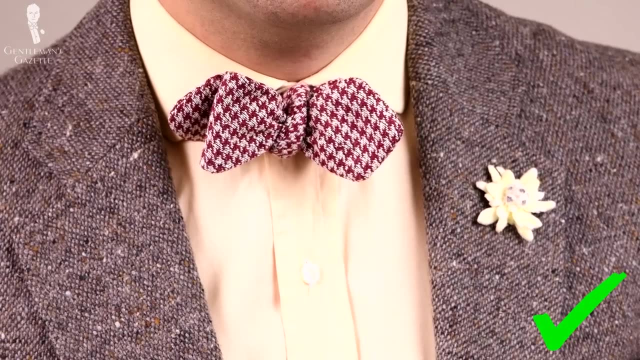 skin tone, so we'll just give a brief overview of it here. If you have light skin and light hair, stick to wearing pastel shades with colors that echo your undertone- Colors like blue, green or purple for a cool skin undertone, and red, yellow and orange. 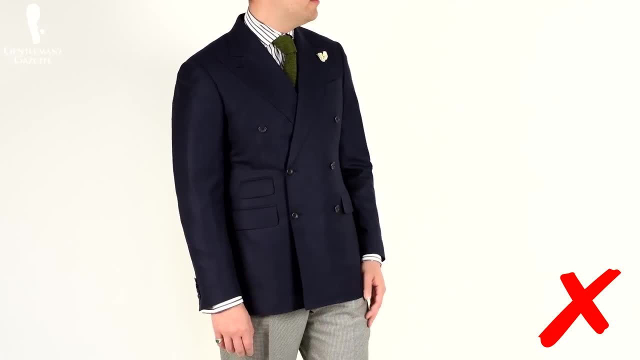 for a warm undertone. Conversely, dark colors and black will most likely make your skin tone a little darker. If you have light skin and light hair, stick to wearing pastel shades with colors that echo your undertone. This will make your skin look washed out and ashen. 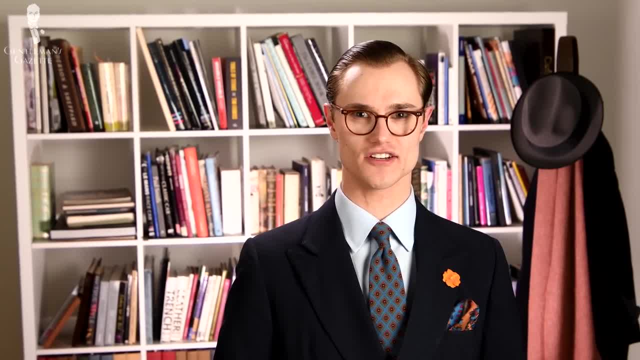 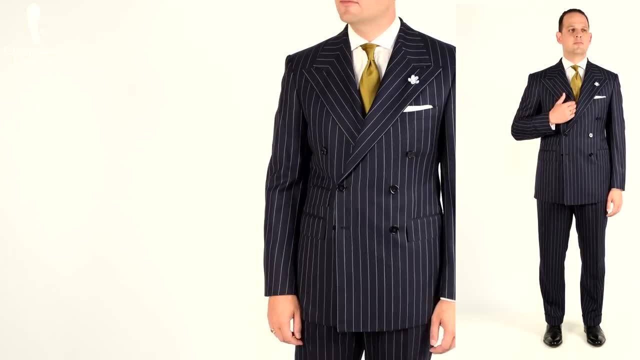 The exception here is if you're a man with light skin and very dark hair, in which case a high contrast man, and then, of course, you can go ahead and wear these darker colors. If you have fair skin and still want to go for a subtle contrast, take a cue from your. 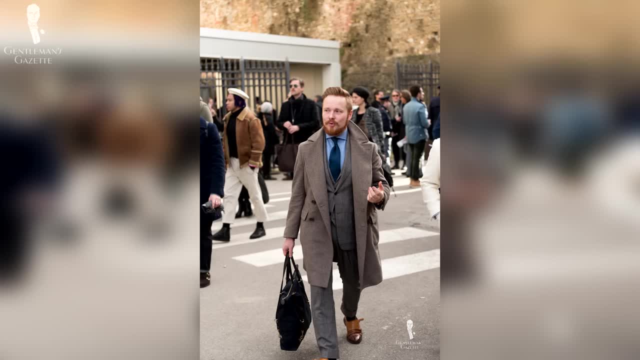 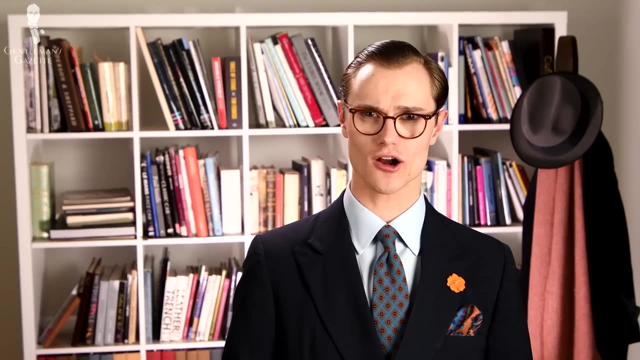 hair color. The classic example here is that red-haired men typically look very good in pastel blue shirts. If you have medium skin and hair, stick to wearing pastel shades with colors that echo your undertone. If you have dark skin and hair, you can start to experiment with more true hues, though be 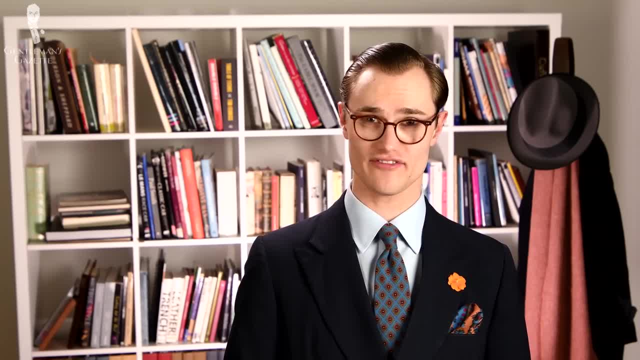 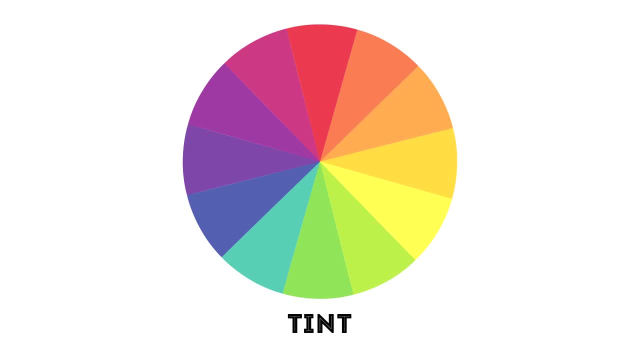 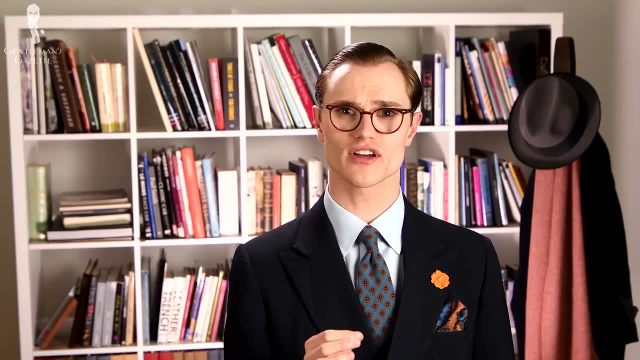 mindful of them and follow the advice that we laid out in the previous section of the video. Slight shades or tints of colors, without being too extreme in either direction, are going to work well for you. You can echo your undertones for a look that's more harmonious, or you can go with the complements. 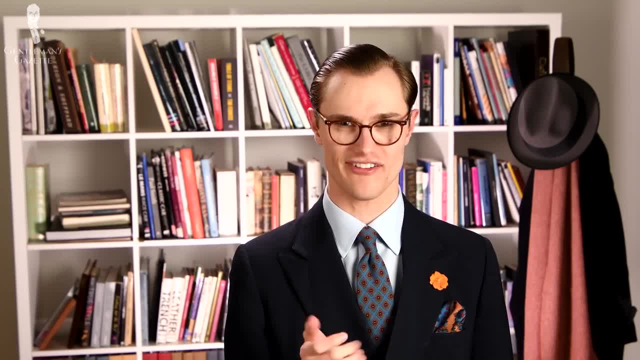 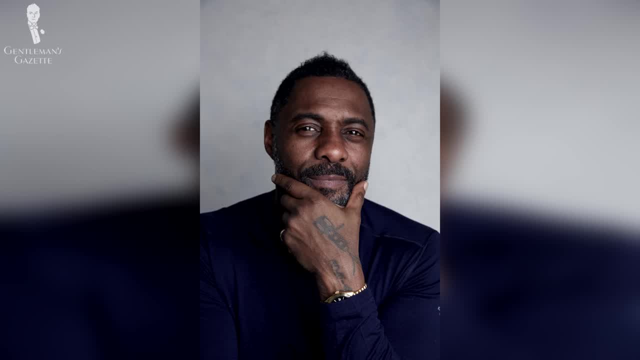 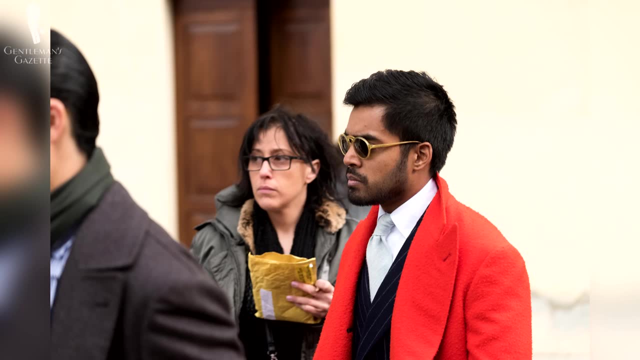 of those colors for something that's a little bit bolder and more fashion forward. Finally, if you have dark skin and dark hair, you're somewhat lucky in being able to wear both true hues and darker shades, as your face is really in no danger of looking washed. 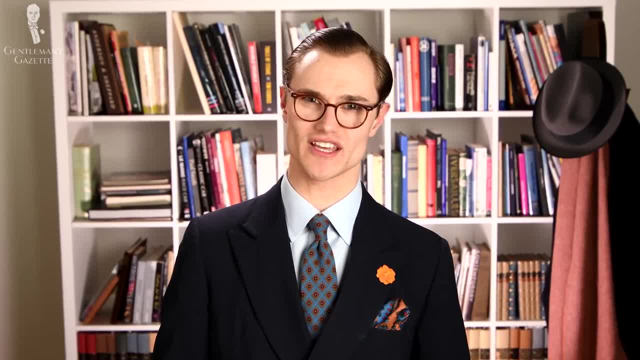 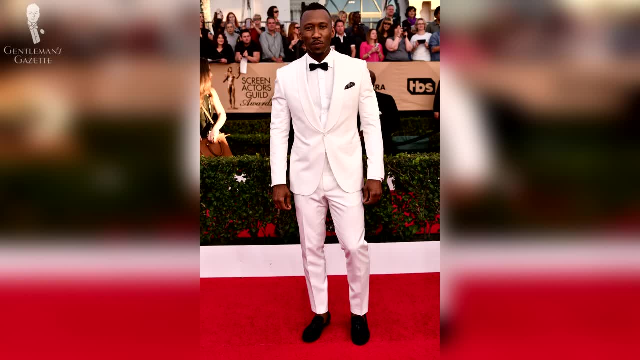 out by these darker colors. The one area to be careful in your position is if you try to wear extremely light tints of colors, as the high contrast will still end up distracting from your face. If you want to wear a lighter garment, we suggest that you try to wear a slightly lighter. 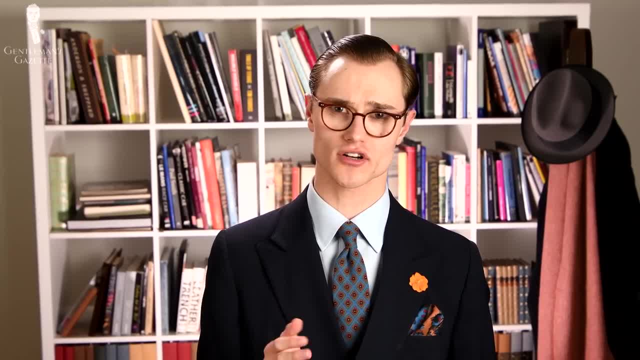 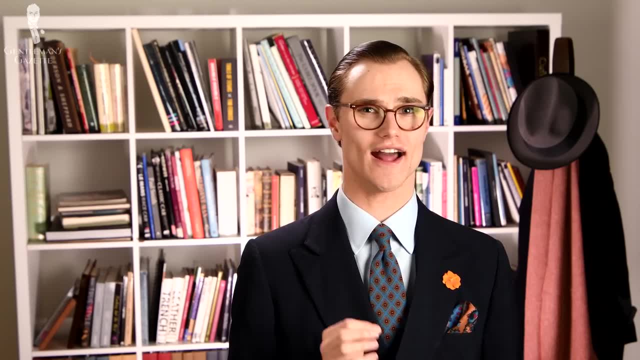 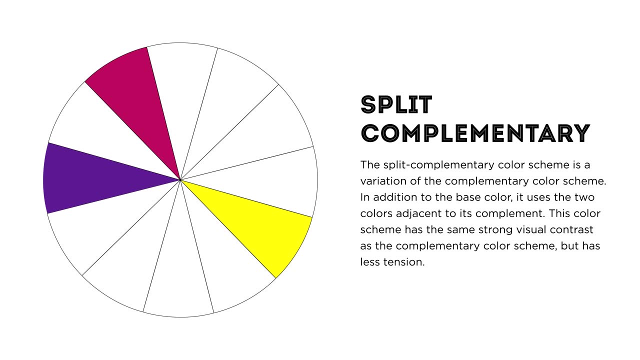 color. We suggest that you do so in conjunction with other darker pieces, As with medium toned men. echo your undertones for more harmony and go with their complements for more contrast. In conclusion, then, knowledge of the color wheel and the broader discipline of color. 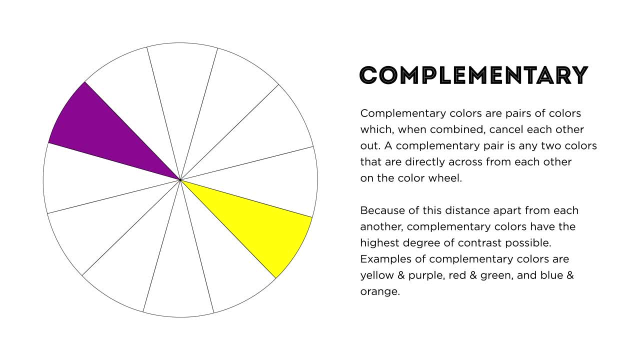 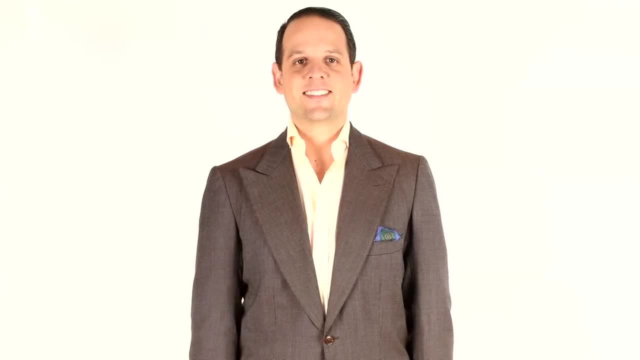 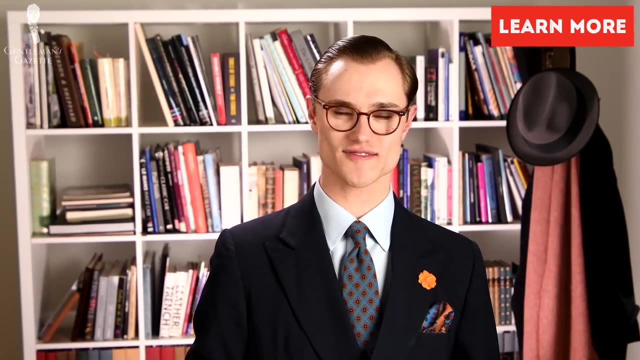 theory is one of the most helpful and versatile tools in the well-dressed gentleman's arsenal. With this knowledge, he can be confident that he's put together harmonious outfits that complement his natural tones and draw proper attention to his face. Also, be sure to check out some of the related articles on our website, such as the article: 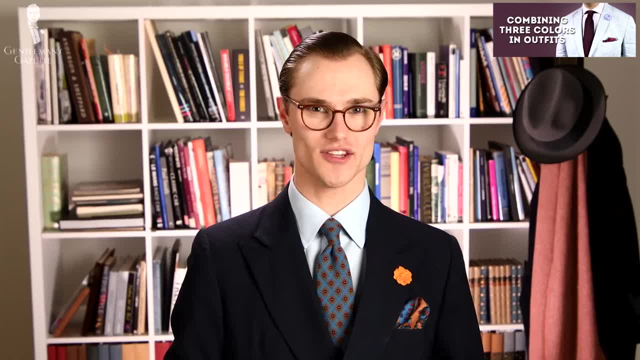 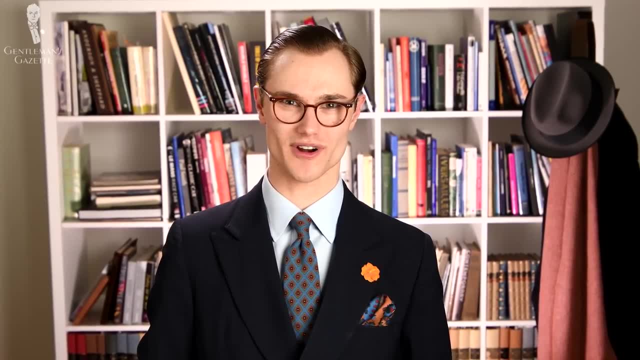 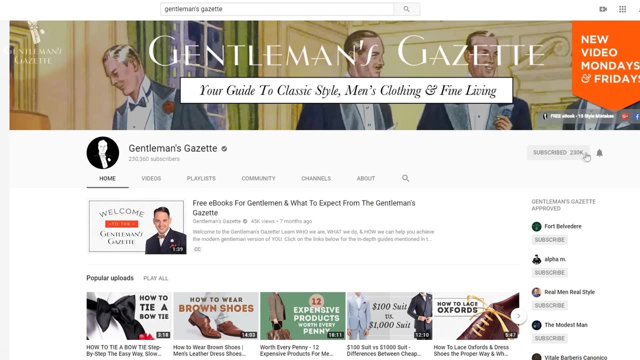 on how to combine three different colors in your outfits. You can find that article by clicking the banner here. So what techniques do you use in order to incorporate color into your wardrobe? Share with us in the comments section below and, as always, don't forget to subscribe to. 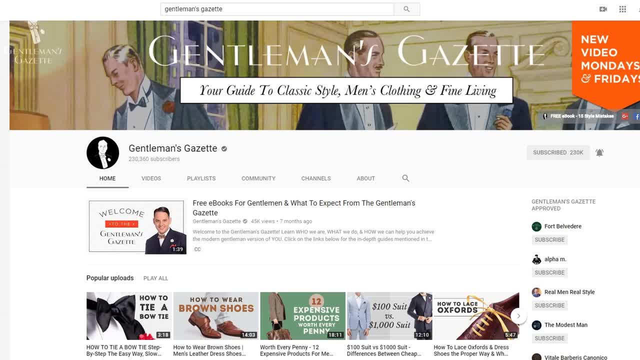 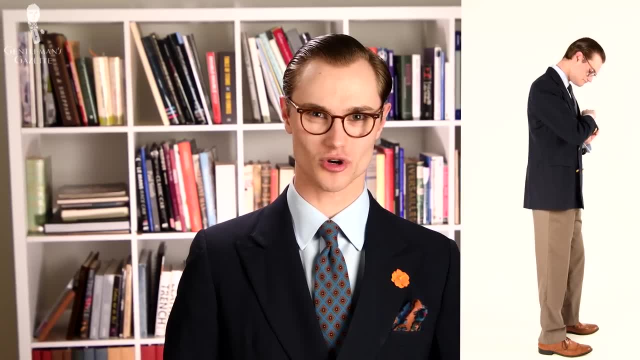 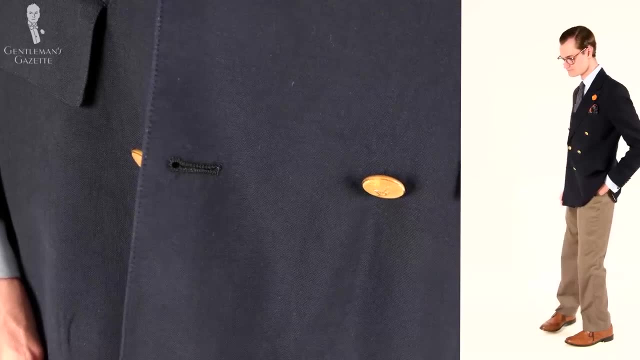 our channel, So videos like these can come straight to your inbox. In today's video, I'm wearing an outfit that incorporates complementary colors, those being blue and orange, of course, in a variety of different ways. My navy blue double-breasted blazer grounds the outfit, but it's light gold buttons as. 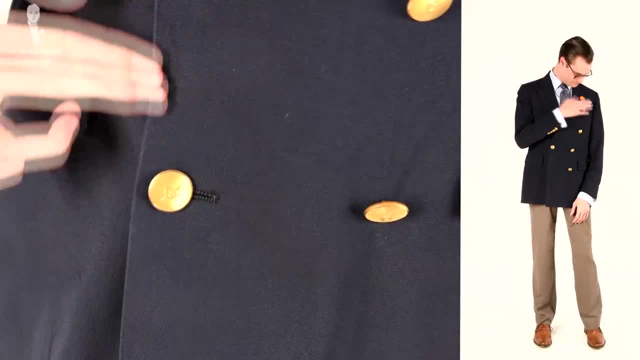 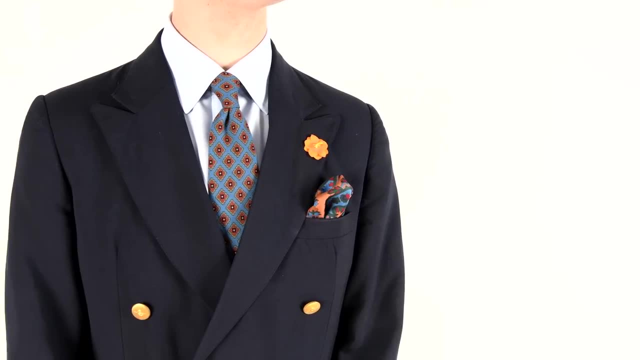 well as some of the other elements in my outfit, make sure that it doesn't wash out my fair skin and medium toned hair. The primary garment helping to lighten my outfit is the navy blue double-breasted blazer. The main outfit is my pastel blue shirt from Charles Tyrwhitt. 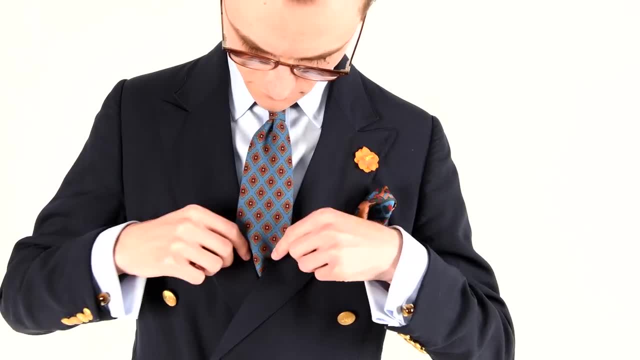 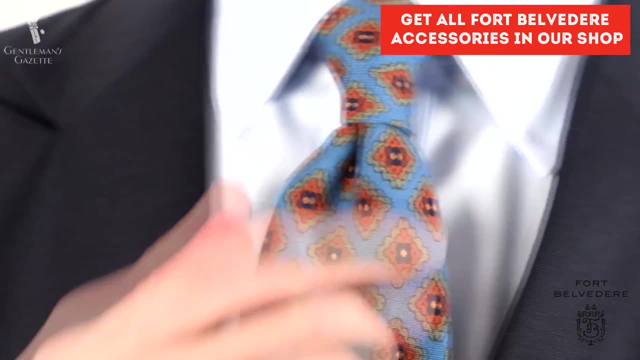 In the middle of the spectrum is my wool chalet tie in turquoise, or would that be blue green that's accented with colors of yellow, gray, orange and navy? This is a tie from Fort Belvedere and you can find it in our shop here. 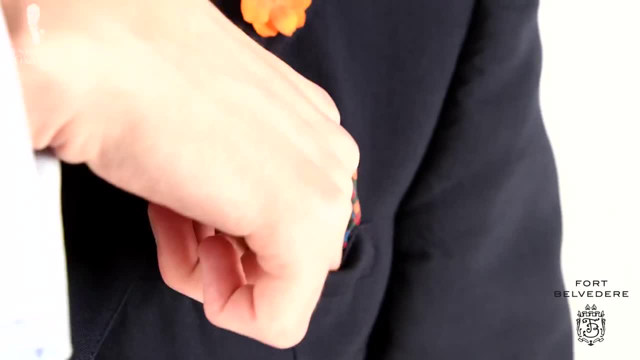 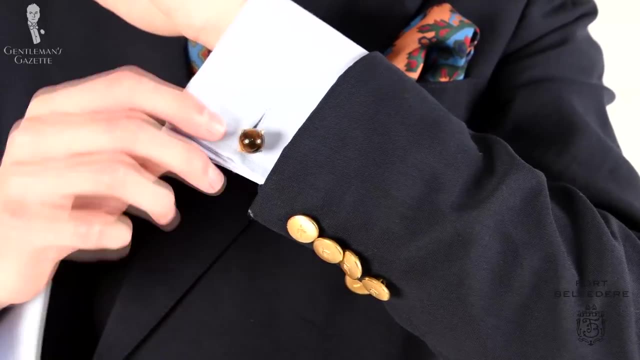 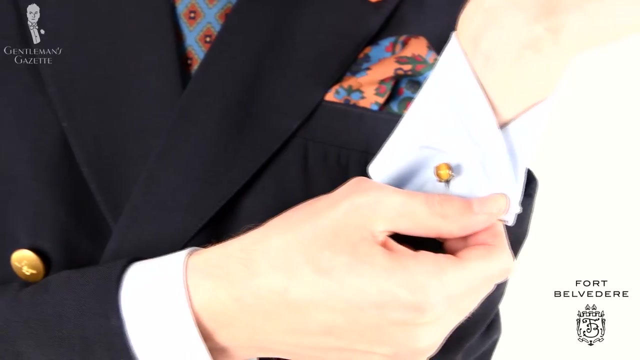 Also featuring a variety of different blue, orange, turquoise and green tones, is my vintage pocket square. This is my vintage pocket square. The accessories also come from Fort Belvedere today, including my gold-plated sterling silver cufflinks. They're in an eagle claw design and they feature tiger's eye as the stone which brings out.